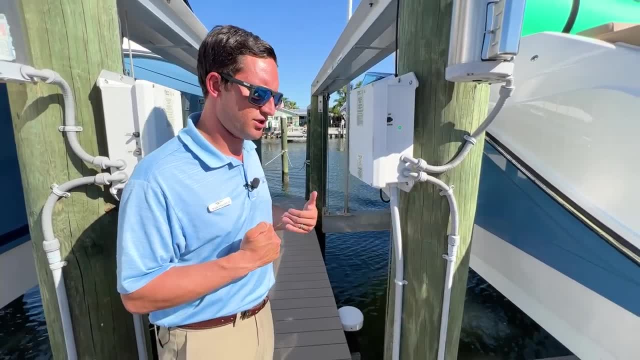 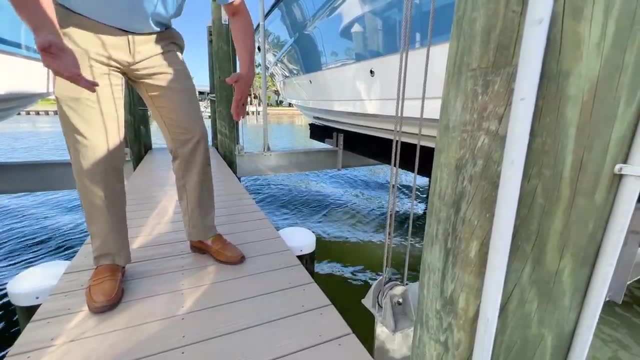 that it's not sitting on any of the chines And how I like to store these boats right here. you notice I have the I-beams right at the dock level. That way, in the event that there is a storm or a storm is going side to side, you have your I-beams hitting your dock and your boat's not really. 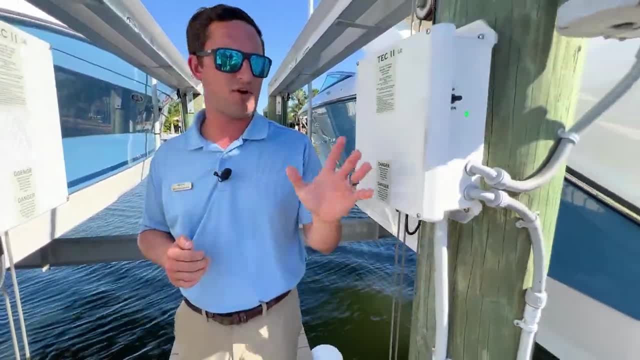 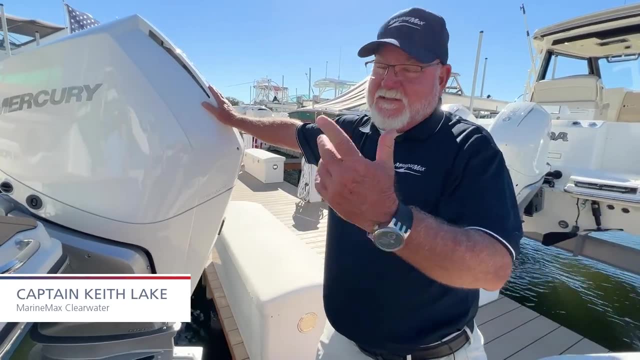 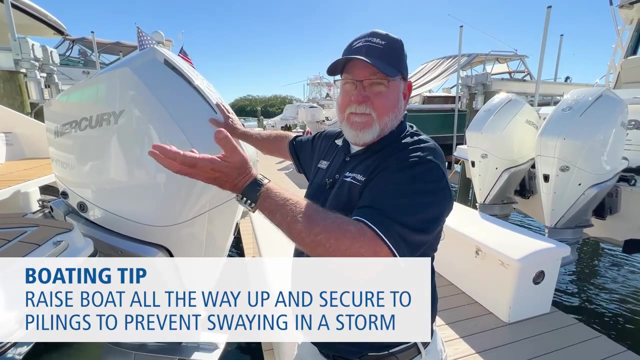 rocking side to side Now you didn't see them earlier. but over here we got captain Keith and Keith's going to go over lift basics 102.. Hey guys, I was just listening to Nick and just coming up with a couple different things. So in a storm you want to raise your boat all the way up? get it up. 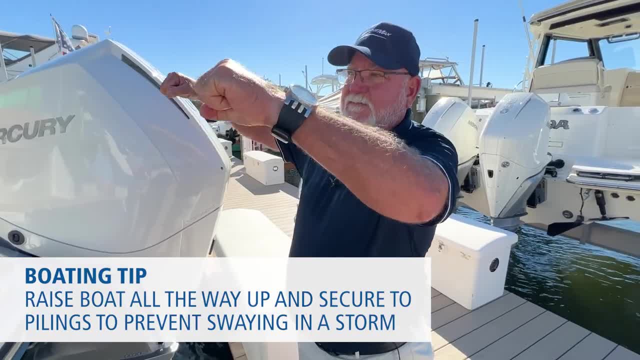 as high as you can safely and then secure the boat and the lift to the to the pilings, because Nick was talking about that swing. Because Nick was talking about that swing, You need to have that lift up to the bottom of the boat. 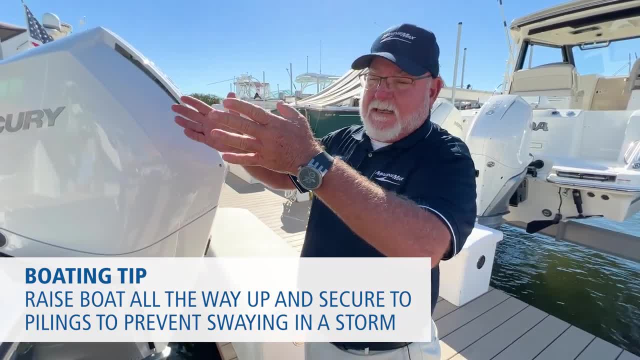 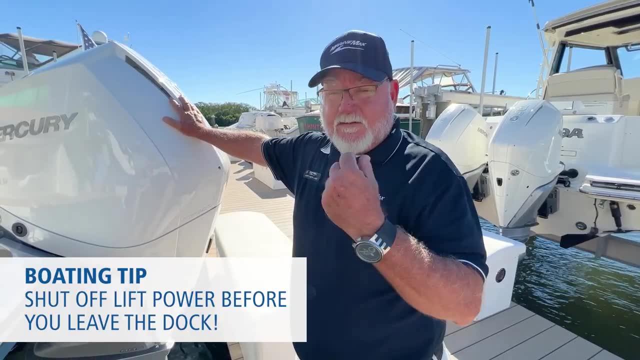 don't want it chewing up your dock, so that'll keep it up. keep it from moving around. Nick mentioned the power to the lift. make sure you shut it off when you're done, at the end of the day, before you leave the dock, because if you take 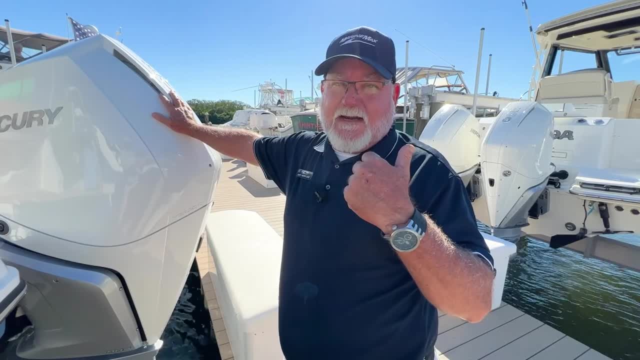 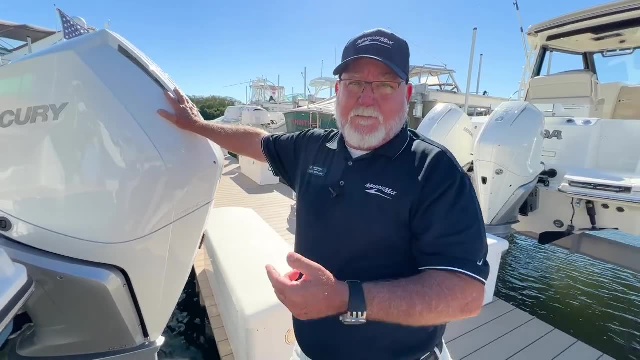 that remote, you stick it in your pocket, you walk up the dock, you go sit down in your house and you sit on that remote, down goes your boat, or maybe bring it all the way up, and then the cables bind up and break when they go up in the top. 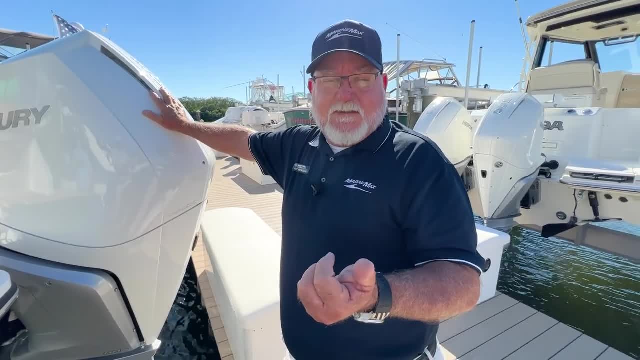 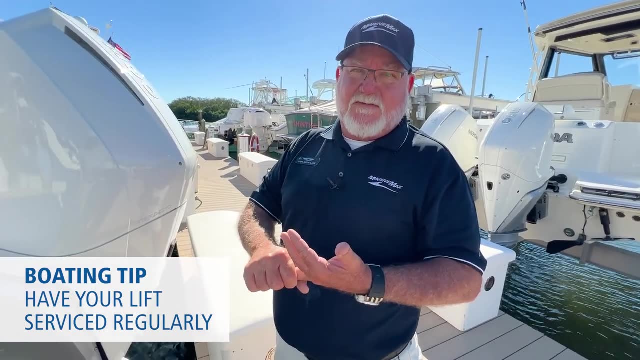 another thing he mentioned about having a reputable lift company come out, have your lift serviced regularly, just like you do your your boats. you know you do the 100-hour service, the annual service. you want to do that. you want to have them check the cables, grease, the fittings and all that stuff, your motor. 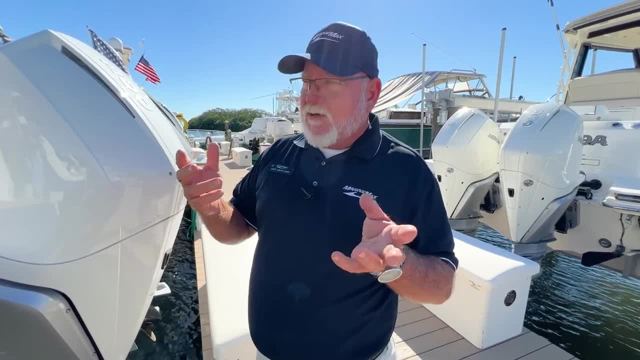 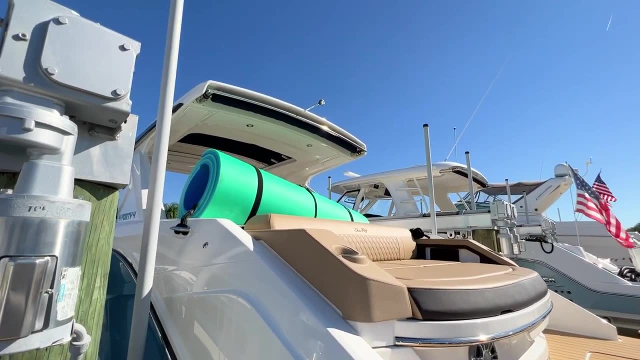 shouldn't be whining and screaming- and then Kelly doesn't know about this, but just something I saw as we stand in here. if you look at the PVC poles, the uprights, so on the bow of this boat, this one's bent over a little bit up there towards. 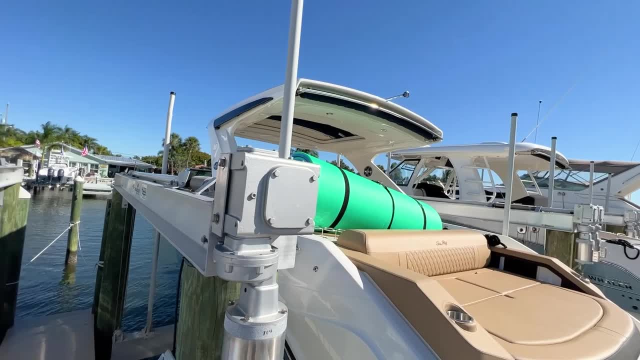 the bottom of the boat, and then the bottom of the boat is bent over a little bit up there towards the bow of the boat and if you look to the boat to his left a little bit, that PVC pipe is snapped off. it's loud too. all right exactly. 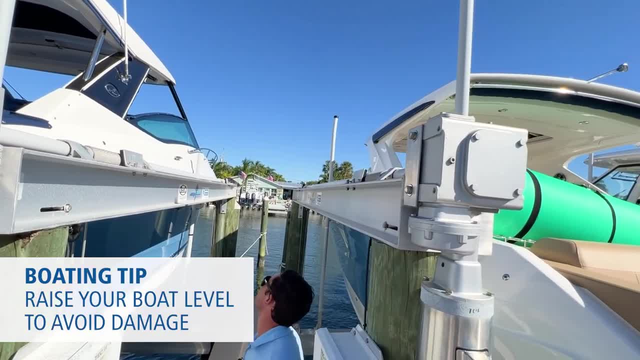 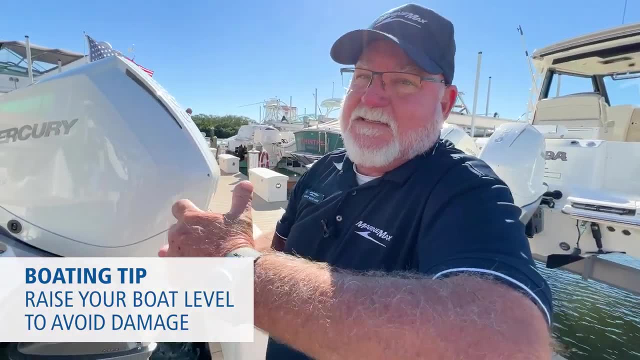 right. so when you're raising your boat, make sure it comes up level and you don't get a cockeyed on there, because if those PVC pipes get hung up underneath those I beams, that thing snaps. it sounds like a shotgun on gun going off right next to your ear. so just watch your poles, watch your uprights when you're.